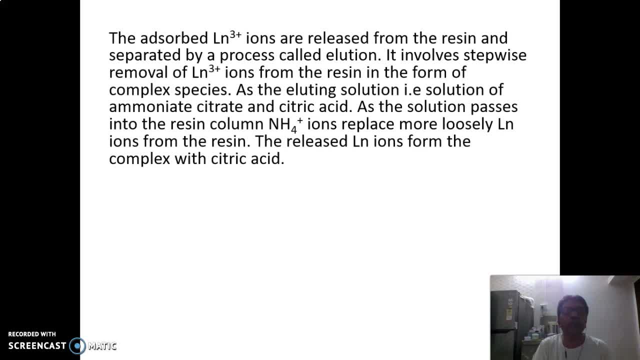 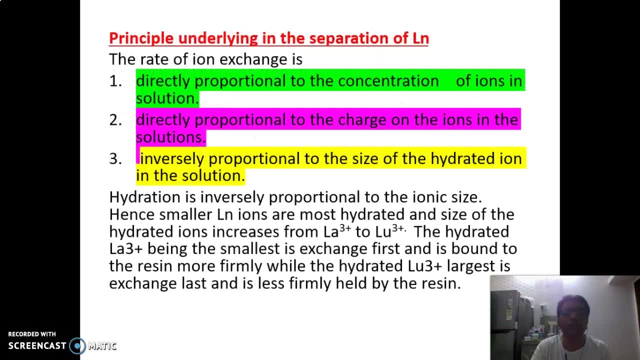 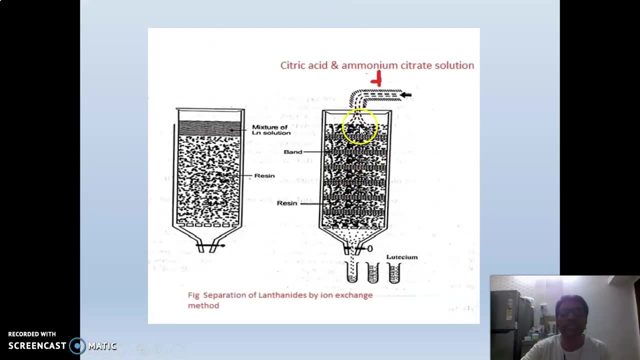 the lanthanum ions in the resin column. the lanthanum ions are absorbed one by one on the resin column in the previous diagram we have shown. so let us see here. so lanthanum ions get exchanged with the resin column one by one, so the 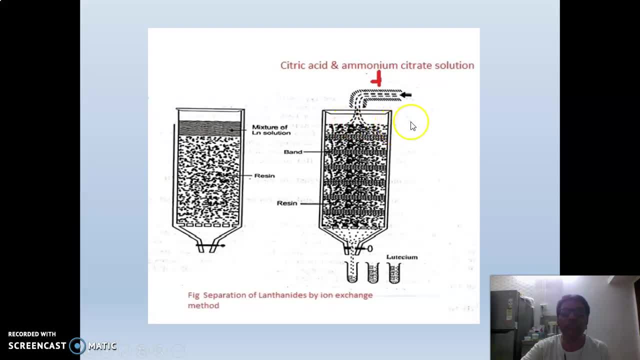 lanthanum 3 plus ion, which is smallest, which has the smallest hydrated radius. it is at the top of the column. lutetium tri-positive ion: it has the largest hydrated radius, which is at the bottom of the column. so in this way the individual separation of the lanthanum ion is takes place. 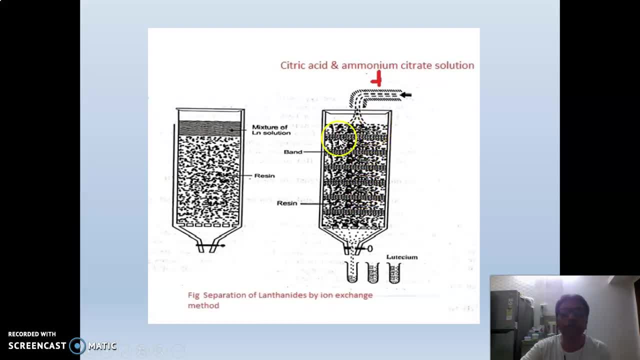 this is the end of the diagram. but now we want to separate and we want to collect the fraction of the lanthanum ions one by one. so the collection and elution of the lanthanum ion is possible only when, by adding a suitable eluent in the resin column in the first step, the 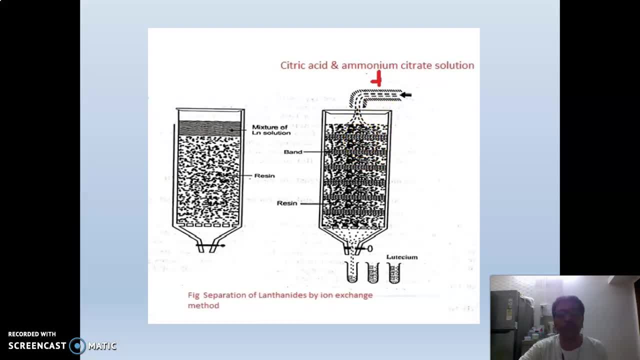 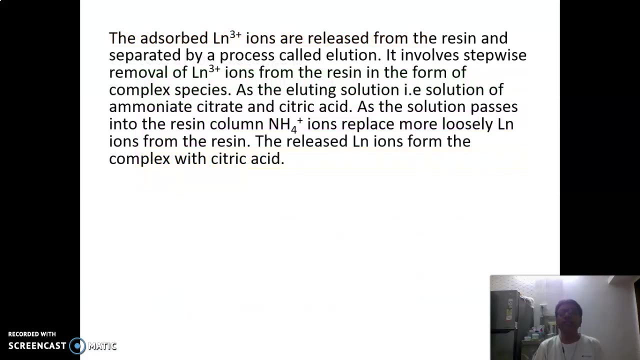 lanthanum ions get attached with the resin column. now we want to separate the lanthanum ions from the resin column by simple elution process. so let us see now: the absorbed lanthanum ions are released from the resin and separated by a process, and that process is called as a elution. so elution involves stepwise. 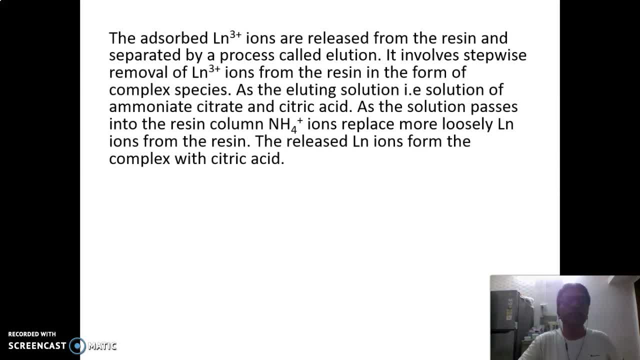 removal of the lanthanum ions from the resin in the form of the complex species, as the elutin solution, that is, the solution of ammonium citrate and citric acid, is added into the resin column. as the solution passes into the resin column, ammonium ion replaces more loosely lanthanum ion from the resin. 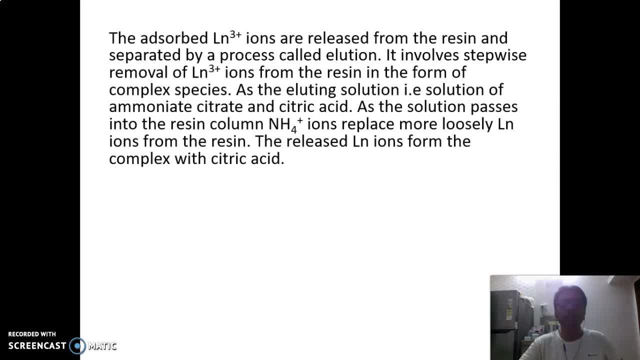 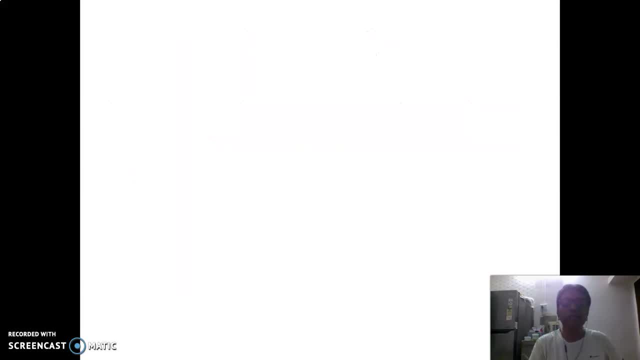 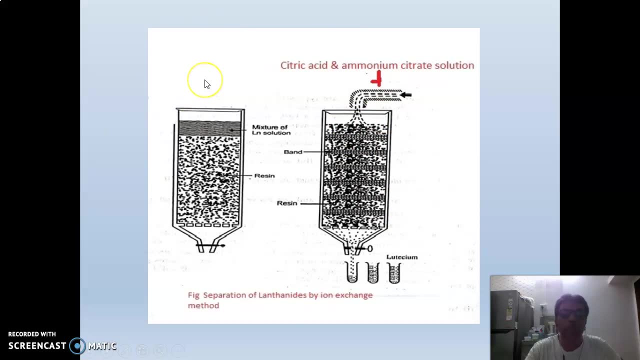 column, then the released lanthanum ion form the complex with the citric acid. once again go to the diagram. I would like to explain this. so see in this diagram. so you have to see here the stirring solution is added into the holder. so the proper solution it is the mixture of citric acid and ammonium. 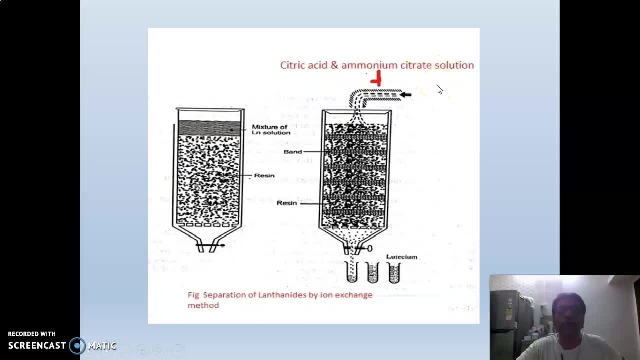 citrate solution, why this join Squid or why this complexing solution is added agent. it is used because this complexing agent gives the better separation factor, so it is added into the resin column. so when the solution of citric acid and ammonium citrate 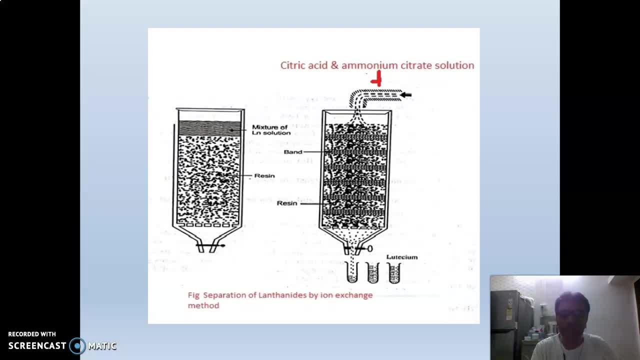 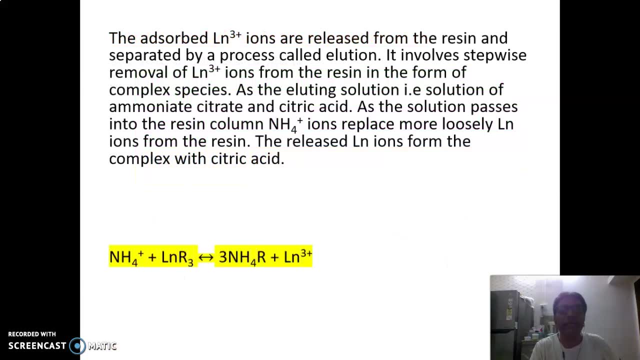 it is added into the resin column, there is a complex formation is complex formation process is takes place and, first of all, when we add the ammonium citrate solution in the resin column, the ammonium ions replaces the loosely held lanthanone from the region and, as we know, lutetium tripositive ion. it is loosely held with the 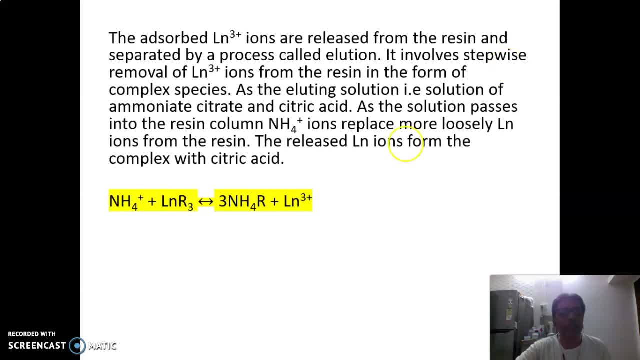 resin column. so this cation ammonium ion replaces the loosely held lanthanone from the resin column. so the ammonium ions get attached. now the resin column and lanthanol ions get free. so one by one the lanthanol ions are released from the region column. one by one the lanthanol ions are. 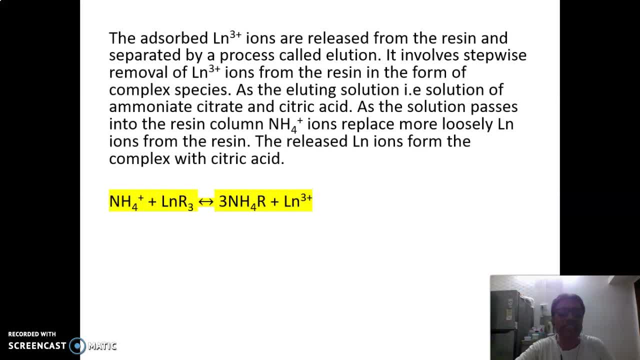 released from the resin column. so in this case also there is a cation exchange process. this happens now second time in the first step, when we add equimolar solution of lanthanol ion in the resin column. lanthanol ions get attached with the resin column, so in that case also there. 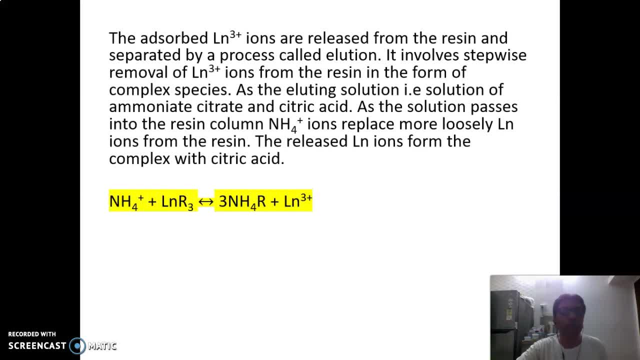 is a cation exchange process. now for the proper separation of the lanthanol ion. when we are adding the eluting solution, that is, solution of ammonium citrate and citric acid, and as the solution passes into the resin, column, ammonium ion replaces the loosely held lanthanum ion from the resin. 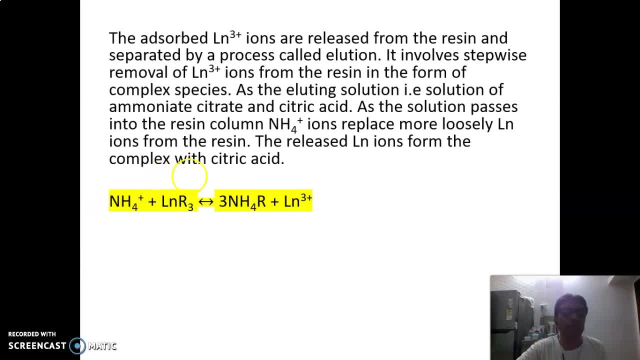 first. so lutetium tri positive ion, it is the loosely held lanthanum ion and it is replaced first. so lutetium tri positive ion, it is released first. okay, see here now the released lanthanum ion. then form a complex with the citrate ion. this citrate ion, it is a. this citrate ion, it is a. 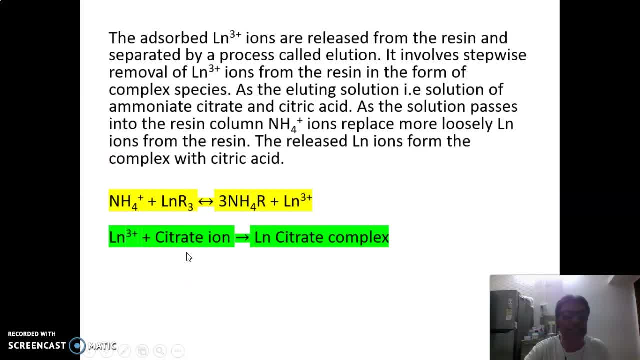 complexing agent. it is a very good complexing agent. citrate ion is a bidentate ligand. it has oxygen atom as the donor atom so it form a stable complex with the lanthanum ion. so the released lanthanum ion from the resin, that is lutetium, tri positive ion. 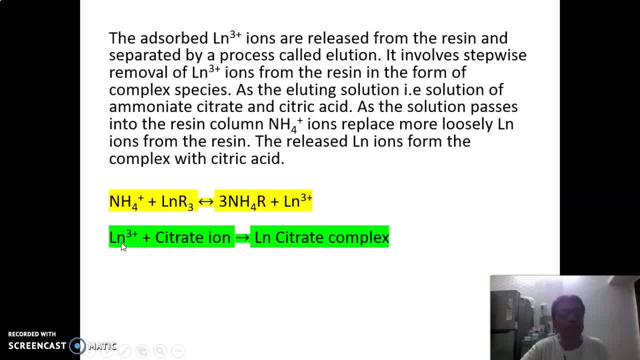 first form, a complex with the lanthanum ion. so there is a lanthanum citrate complex is formed. so this is a very important step. so in this way, one by one, there is a complex formation process is takes place. first, complex which is formed, that is, a complex of the lutetium. 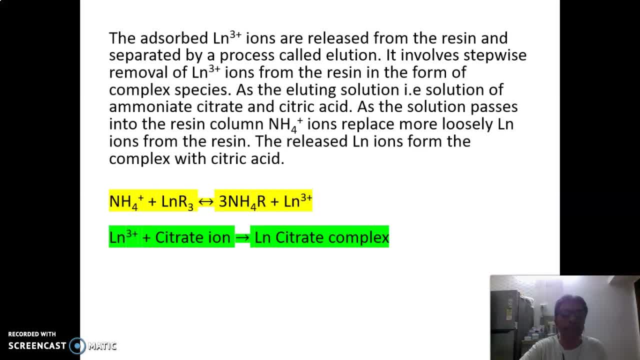 with citrate ion and the last complex which is formed, that is, the complex of the lanthanum ion with the resin column. so in this way the individual separation of the lanthanum is takes place. okay, so at the top of the column the lanthanum citrate complex get formed and at the bottom of the 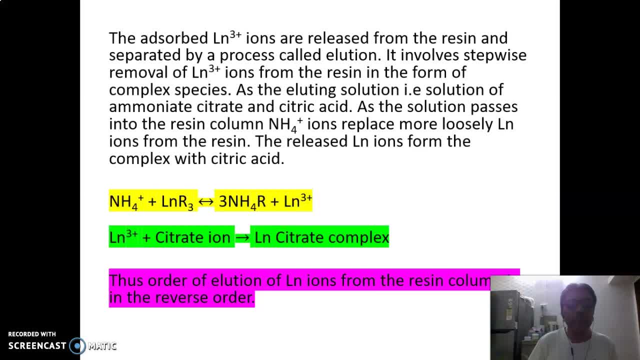 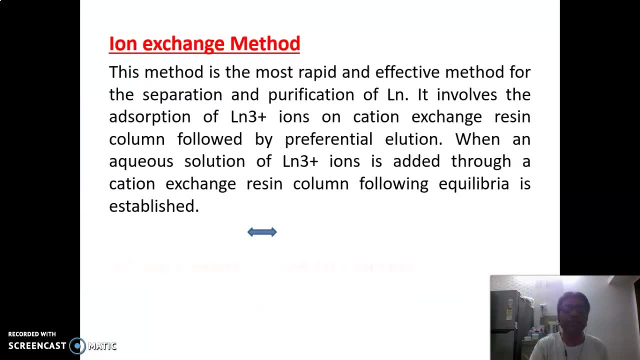 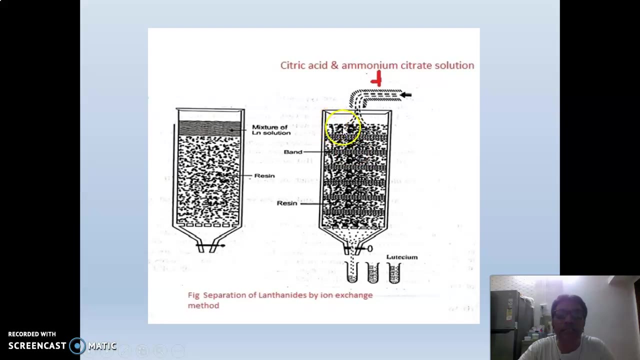 resin column, the complex of the lutetium ion get formed. so in this way the individual bands are created in the resin column. okay, let us once again show in the diagram the individual bands are created there. so you can see the individual bands are created here. so this is the complex of the lanthanum tripositive ion with citrate ion. 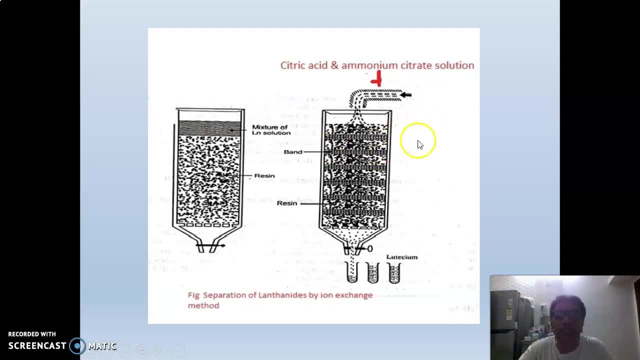 then cerium tri positive ion with citrate ion. so cerium citrate ion complex is formed. and last one that is at the bottom of the column, it is lutetium tri positive ion with the citrate ion. so in this way individual bands are created here. 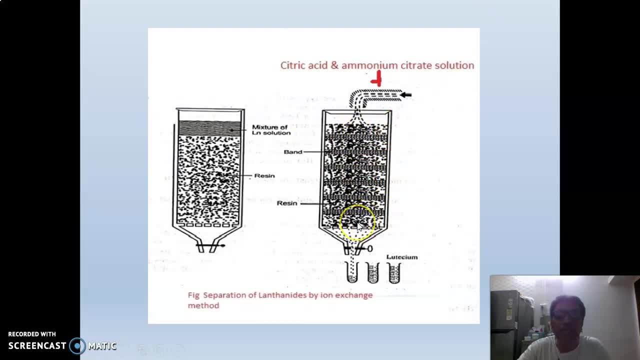 in the resin column. okay, so at the last, uh, at the bottom of the resin, uh, at the bottom of the resin column, the lutetium tri positive ion is here. the complex of the lutetium tri positive ion is here, which is a very stable complex, because the ionic size of the lutetium tri positive 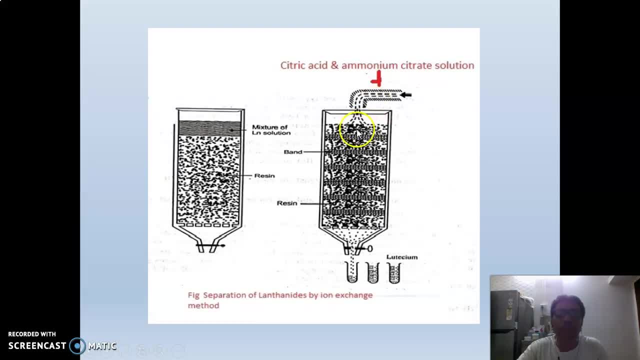 ion is smallest and the lanthanum tri positive ion which is at the top of the resin column, so it is somewhat less stable, complex, as compared to the lutetium tri positive ion, complex. so in this way individual separation of the lanthanum ion is takes place here and one by one we can collect the fraction. 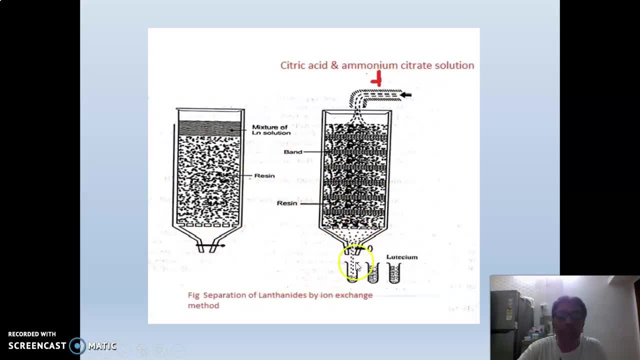 of the lanthanum ion. okay, so first fraction which is collected, that is glutathione. second fraction which is collected, that is ytterbium. third fraction that is collected, it is thulium. so, in this way, the last fraction which is collected, it is lanthanum tripositive ion. 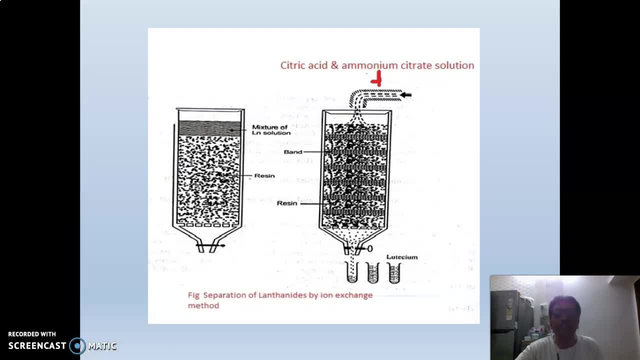 so these ions are separated from each other in this way. so in the separation of the lanthanum, complexing agent plays a very important role. when we add the solution of the complexing agent, that is, citric acid and ammonium citrate solution, it creates the individual bands in the resin. 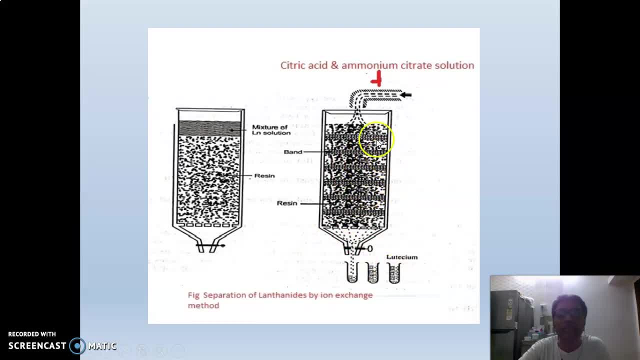 column. not only it creates the individual band in the resin column, but also it increases the cation exchange capacity of the resin column. okay so, and it also gives the very good separation factor. separation factor plays a very important role in the separation of the lanthanum. if the separation factor it deviates from unity, then the proper separation of the 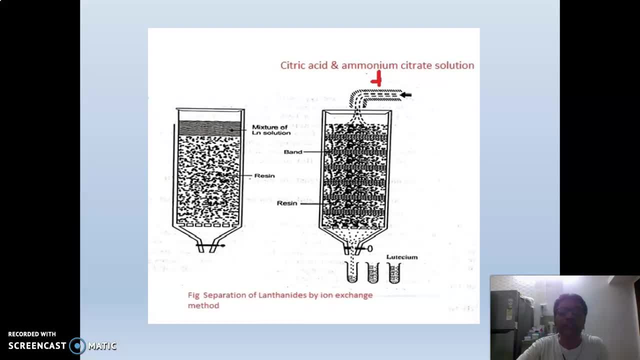 lanthanum ion is takes place. okay, so once again i would like to explain here how the lanthanum ions are separated from each other. first step- it is here- the preparation of the resin column. now, once the resin column, it is ready for the separation of the lanthanum ion. 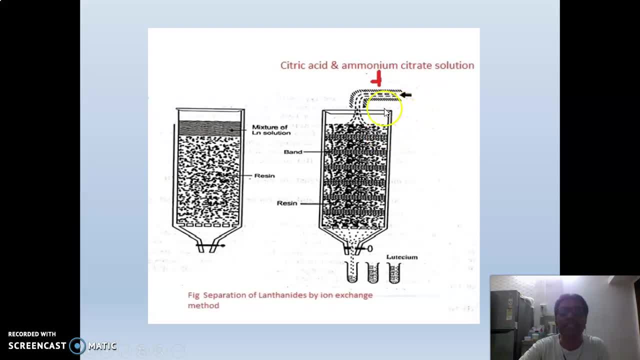 then the solution of the lanthanum ion. it is added equimolar solution of the lanthanum ion. it is added into the resin column. okay, so lanthanum ions are exchanged with the resin column one by one. it depends upon their hydration radius. okay, so the lanthanum ion which has a largest hydrated radius, it gets exchanged. 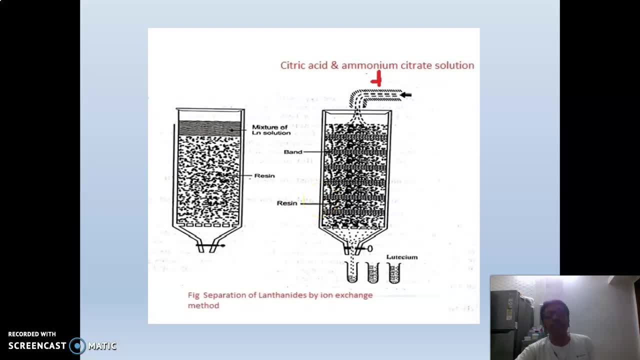 with the resin column and the lanthanum ion, which is which have a smallest hydrated radius. it is exchanged last with the resin column. so in this way, lanthanum 3 plus ion- it is at the top of the resin column- and lutetium tri positive ion- it is at the bottom of the resin column. so the lanthanum 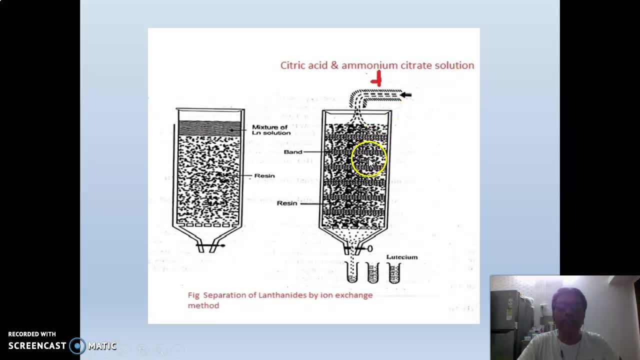 ion is at the top of the resin column and lutetium tri positive ion it is at the bottom of the resin column here. okay, now we want to release the lanthanum ion from the resin column, so eluent should be added into the resin column. actually, acidic solution can be added, but it it cannot use the good separation. 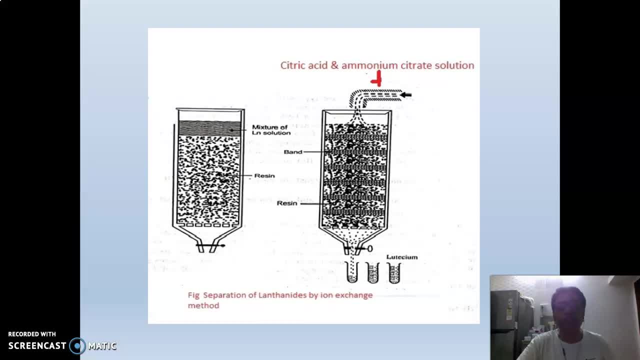 factor and individual separation of the lanthanum ion is not possible. so therefore, in the separation of the lanthanum ion, the proper eluent it is to be added, so this citric acid and ammonium citrate solution. it is added into the resin column and it create the individual bands of the resin. 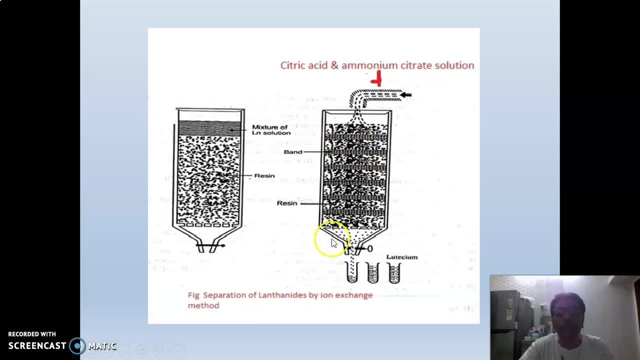 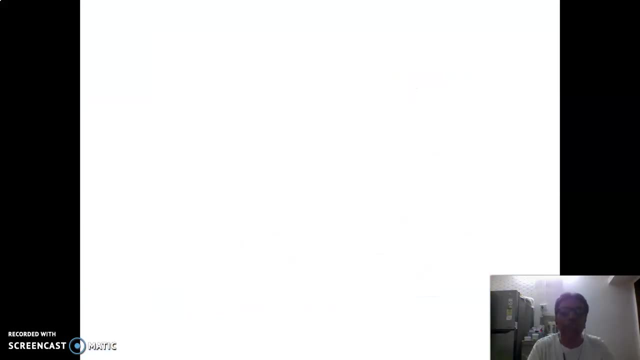 column. there is a complex formation process is takes place here. okay, so citric acid, citrate ion. it is a complexing ligand and it is forming the complex with the lanthanum ion. okay, so let us once again show the equilibria which is established in the separation of the lanthanum ion. so see here. 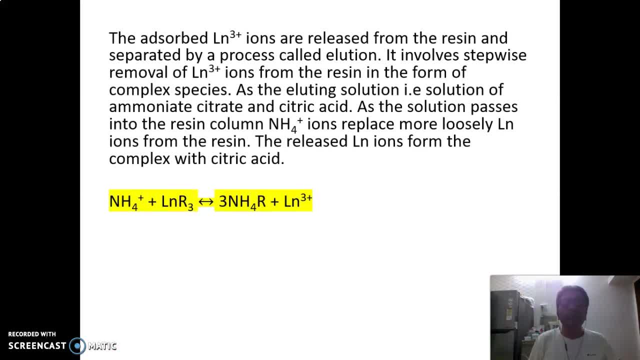 when we are adding the solution of citric acid, ammonium citrate, into the resin column. the ammonium ions replaces the loosely bound lanthanum ion with the resin column and that is lutetium tri positive ion. so one by one the lanthanum ions are released from the resin column again in this. 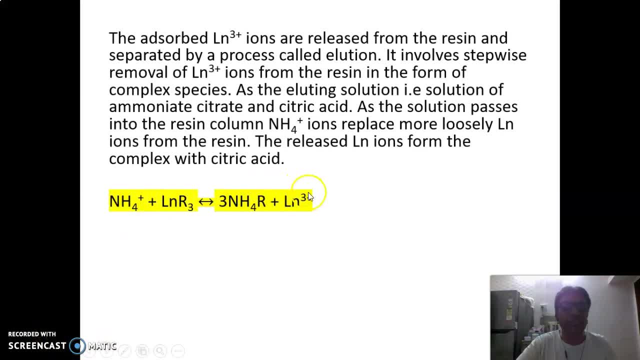 case cation exchange process is takes place. okay, so lutetium tri positive ion is released first and it is going to form the stable complex with the resin column here. so the stable complex of the lutetium tri positive ion with citrate ion gate form here. so that is the lutetium citrate complex. 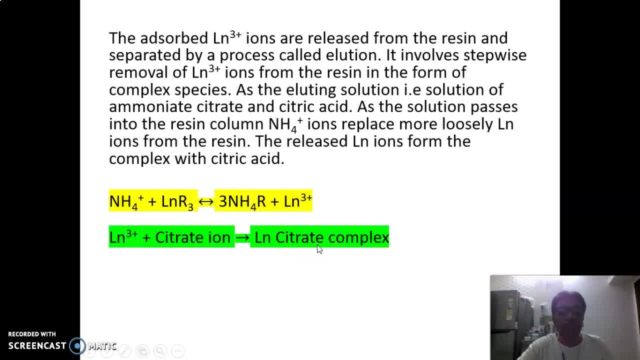 or lanthanum citrate complex. it is formed here, okay. later on other lanthanum ions are also going to form the complexes with the resin column. okay, so one by one, there is a complex formation process is takes place in the resin column. so the second area is the awaken. that usually looks more clear, even if it looks outside, and we can. 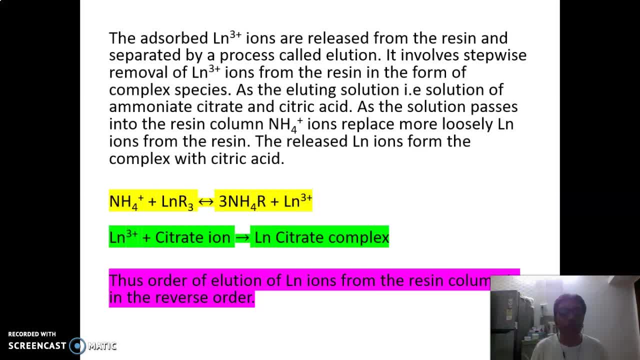 understand other levels better, a bit more clearly now. this is really a complex configuration. so we can imagineícios of the yellow fan joining with tan ils and dancing on them or living on them. uh, in this, qual skullea baixa. so some of these possibilities exist, that. we are going to study another time, so we will get the lutetium tri positive ion, which is the main at the top of the column, and lutetium tri positive ions, which is remain at the top of the column, and lutetium tri positive ions, which is remain at the bottom of. 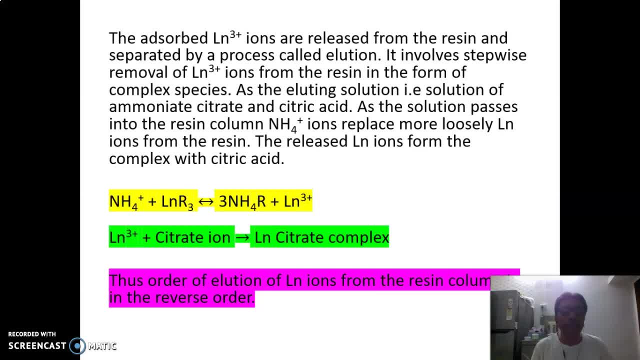 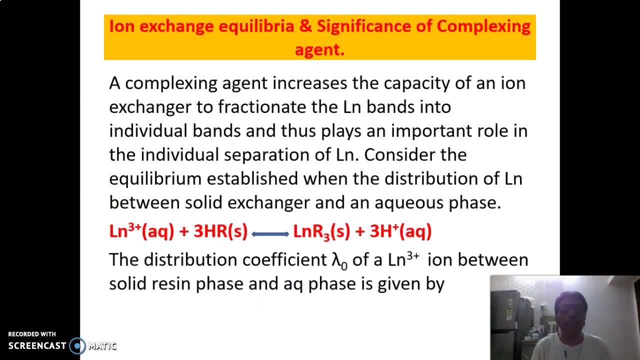 lanthanum tripositive ion. okay, so in this way the elution order it is in the reverse manner: lutetium tripositive ion come first, then the lanthanum tripositive ion come last during the separation of the lanthanum ions. okay, so in this way the lanthanum ions are separated from each. 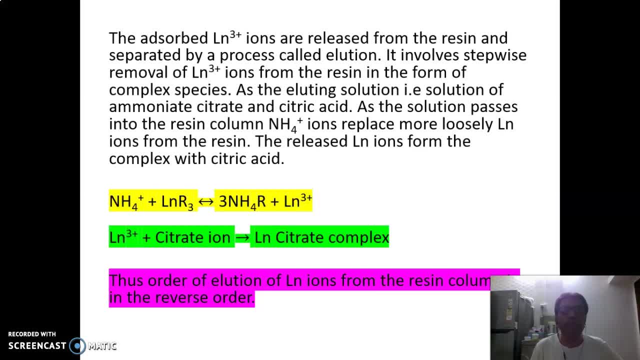 other. so this is the ion exchange method which explain the separation of the lanthanum ion from each other. so the individual separation of the lanthanum ion is possible with the help of the ion exchange method. this method is very rapid method. this method is very effective method for. 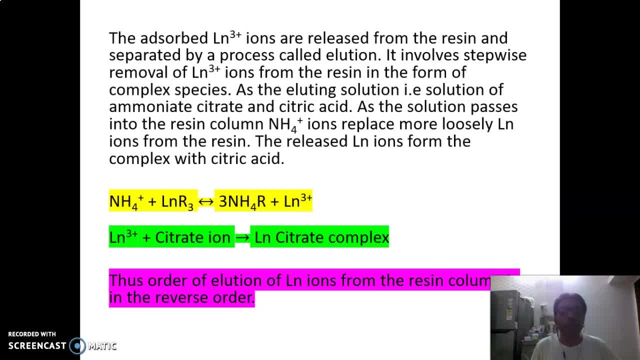 the separation of the lanthanum ion. so try to understand how the lanthanum ions are separated from each other.